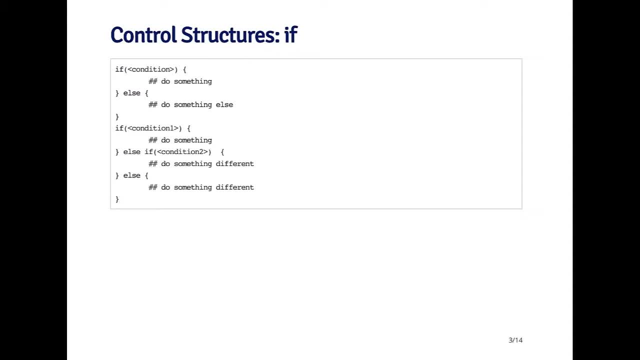 So if the condition is true, then you do something else. you do something else. That's a typical kind of construct. The else part is optional, so you could just have an if statement to do something if something is true, but you can have the else part if you want to do something alternatively. 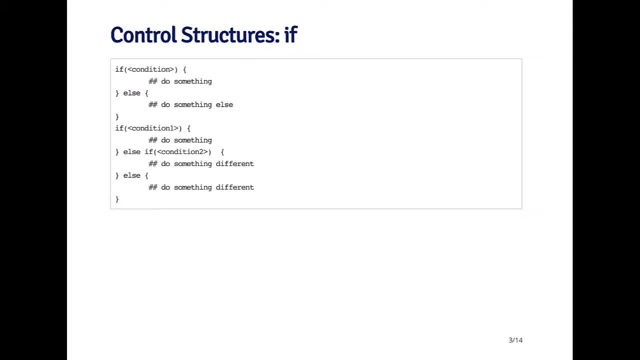 If you want to do more, if there's more than one possible type of condition, you can test. you want to check, you can say if and then else, if and then else Else, if there can be any number of else if conditions in a construct like this. 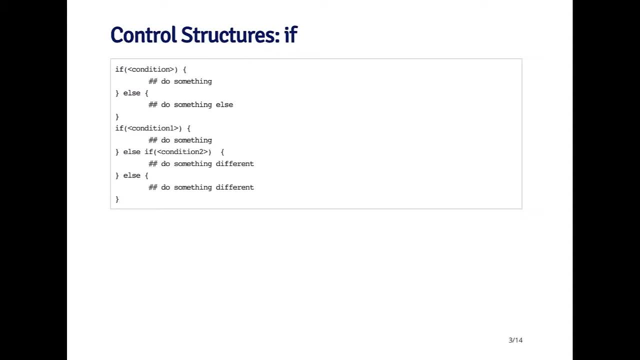 and the else one has to be at the end. So there are a couple of different ways that you can formulate the if else construct. in R It's a little. this is a little bit different from other languages. in case you haven't seen something like this: 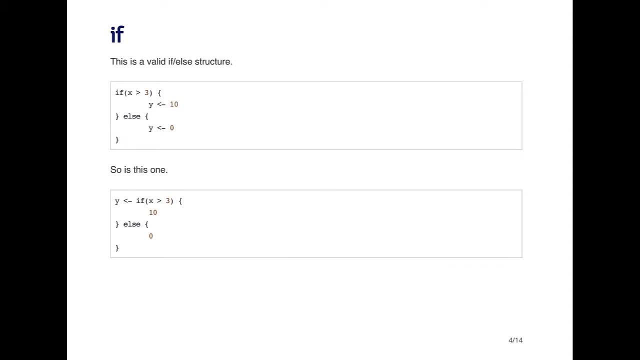 So the first is pretty standard. If x, if the- sorry, if the symbol x is greater than three, then you select, you set y equal to ten. If it's not greater than three, then you set y equal to zero. 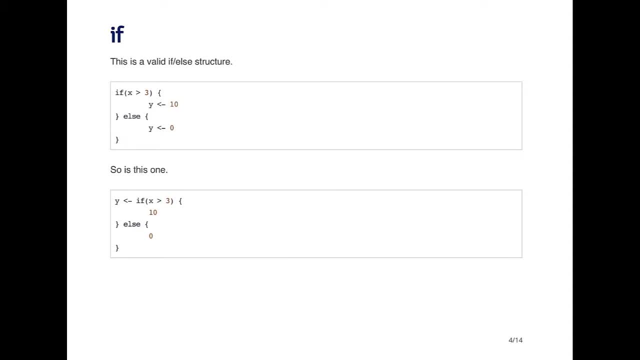 So that's inside the if else construct there's, there's an assignment of y to a specific type of value, depending on what the value of three of x is. But however, in R you can do it a different way. You can say: y is equal to the entire if else construct. 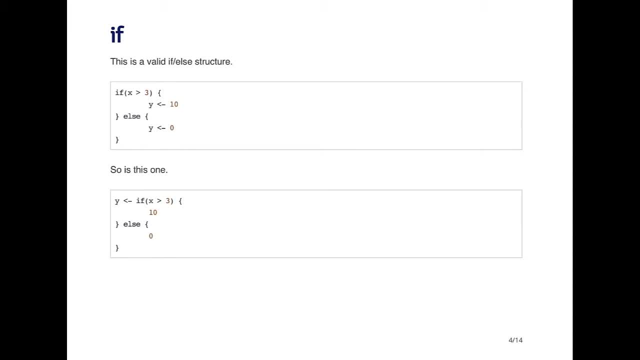 So if x is greater than three, ten or zero, depending on whether that condition is true or not. So this is a valid formulation. also, Sometimes it's it's useful to read this type of writing, because it allows you to realize that the entire if else construct is all about assigning a value to y. 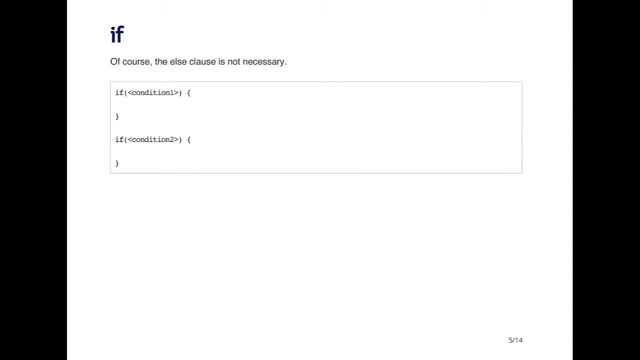 So, as I said before, the else clause is not really necessary. You can always test a condition and do something and do, and then do nothing if that condition happens to be false. So you can, and you can just test multiple conditions in a row if you want. 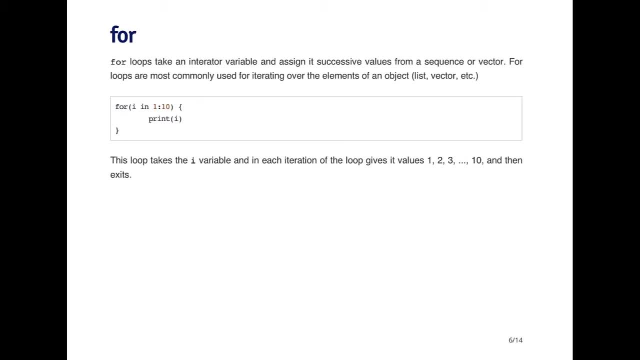 So the next contract is a for loop, So this is probably the most common type of loop operator that you're going to use In R. The basic idea is that you have a loop index, which is typically called i, But if you have many loops, 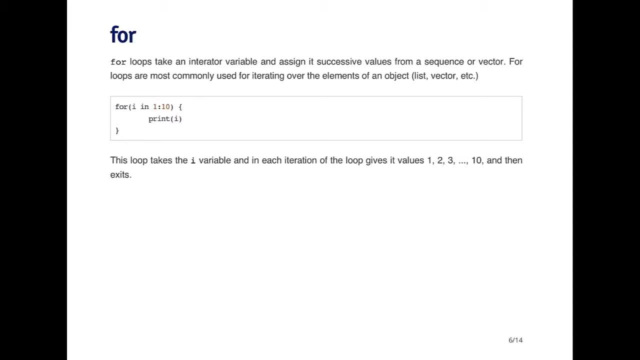 you might say j, k, l, etc. And a loop index is going to go from. it's going to cover a sequence of numbers, typically in integers. So, for example, here I've got a for loop And it's looping over the numbers one through ten. 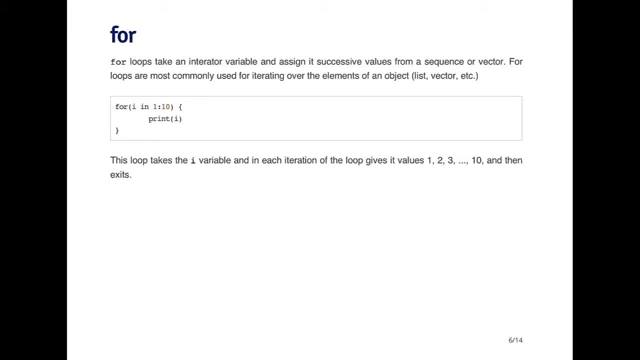 So I've created the sequence of the colon operator, one through ten, And this for loop is not doing anything particularly interesting, It's just printing out the numbers. So I'm printing out i at each iteration. After the loop is finished, it continues on to the next block of code. 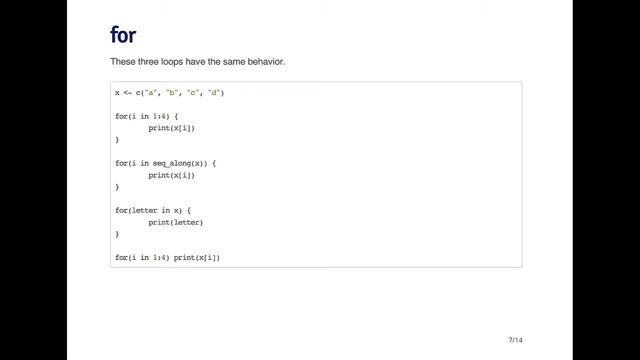 So there's different ways to use a for loop And R is pretty flexible about how you can kind of index the different types of R objects. So here I've created a vector, a character vector, with the letters a, b, c. 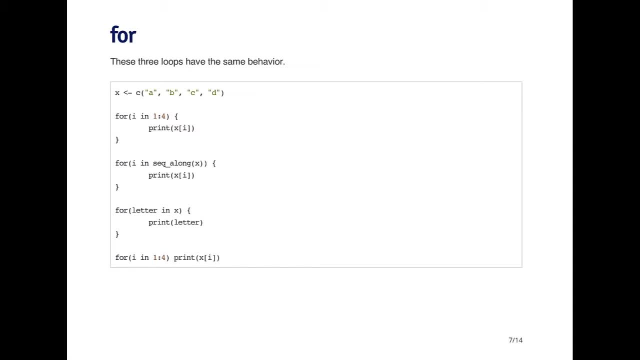 d in it And all of these for loops are equivalent. So for example, the first one, I kind of done what you might commonly see in other languages like C that have for looping. Here I've got an index i that I sequence through one through four. 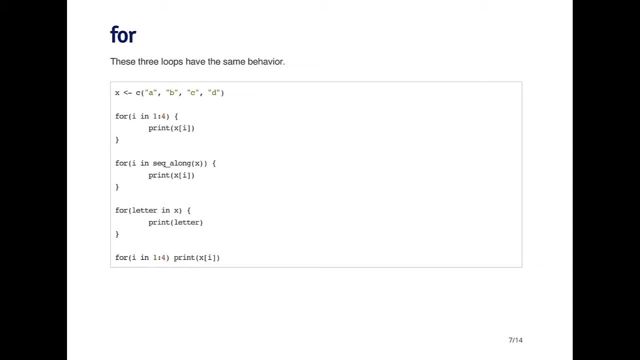 I create an integer sequence And then I print out the ith element of x each time. So here this loop just prints out a, b, c, d. Another thing I can do is use the seek along function, So seek underscore along. 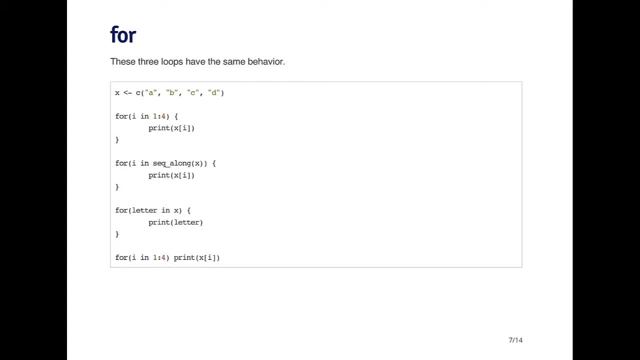 What it does is it takes a vector as an input And it creates an integer sequence that's equal to the length of that vector. So this is a vector of length four. So it's going to create an integer sequence One through four. 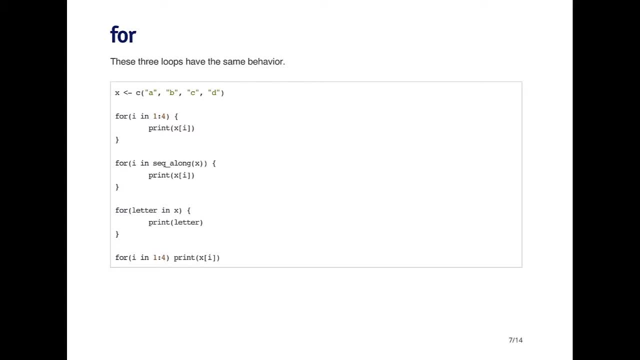 It's exactly the same as the previous statement where I've got the sequence one, colon four. However, here I generate the sequence based on the length of the variable x. So now my index variable. i is going through this sequence. It's printing out the ith element of x. 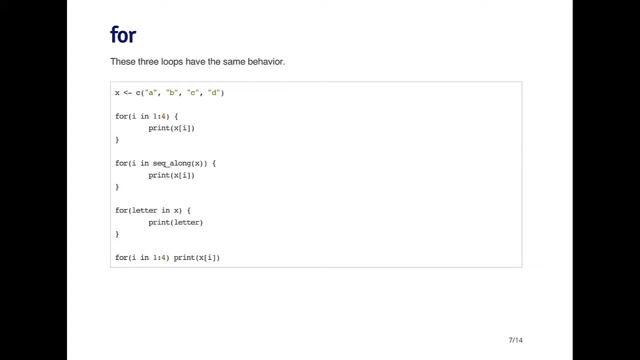 And exactly the same behavior occurs. I print out a, b, c and d. The third example: here I've got a different index variable, I'm calling it letter, And the index variable is actually going to be integer And the index is going to be taking values from the vector itself. 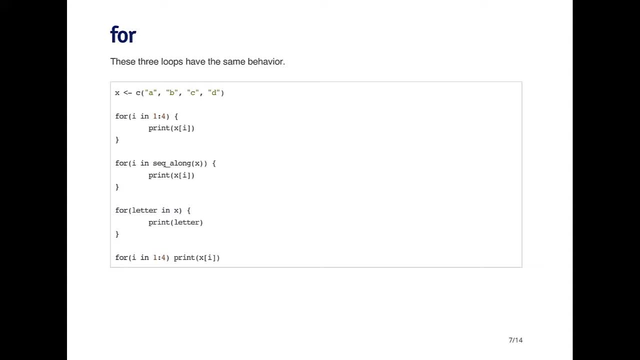 So there's no reason why the index variable has to be an integer. It can take elements from any arbitrary vector. So now the for loop is going through this vector of letters a, b, c, d, And it's just going to print out the letter itself. 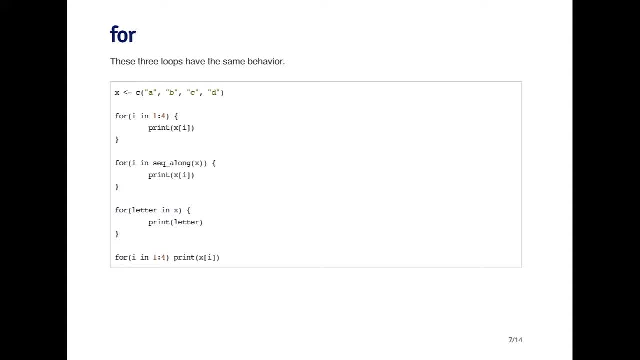 So now I'm printing out the index variable, which happens to be equal to the letters in the vector, And so these three for loops are exactly the same. so far, The last version here is the same as the first one, Except I haven't included the curly braces. 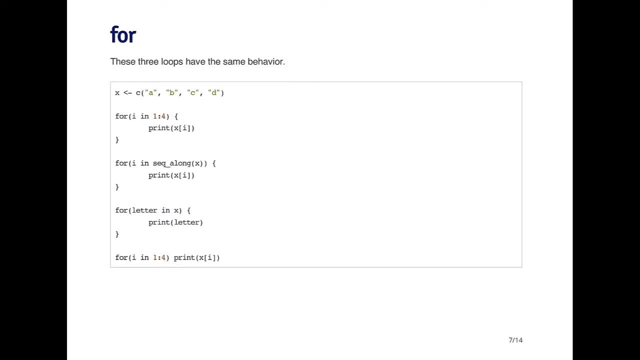 And so for a single expression. if the for loop only has a single expression in its body, you can omit the curly braces and put everything on one line, Which may be useful sometimes because it's a little bit more compact, But it's not my particular style. 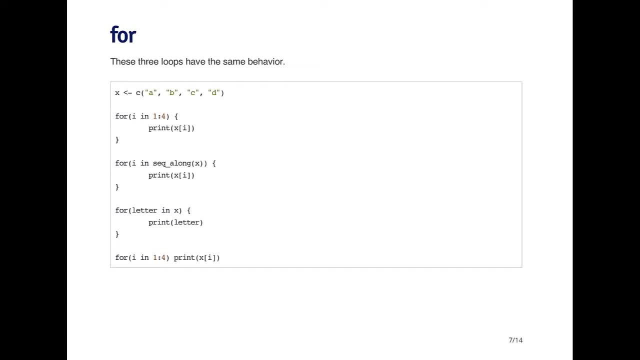 For for loops. I generally like to put the curly braces in. regardless of how many elements are in the body, For loops can be nested So you can have a for loop inside of a for loop. So the common thing, for example, is with a matrix that has two dimensions. 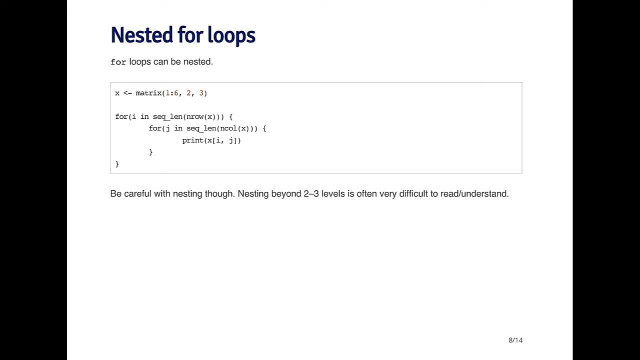 And then you might want to loop over the rows and then loop over the columns. So here the outer loop with the i index is looping over the rows And I'm using a function that's called seek underscore len. So the idea is that it takes the seek underscore len, takes an integer. 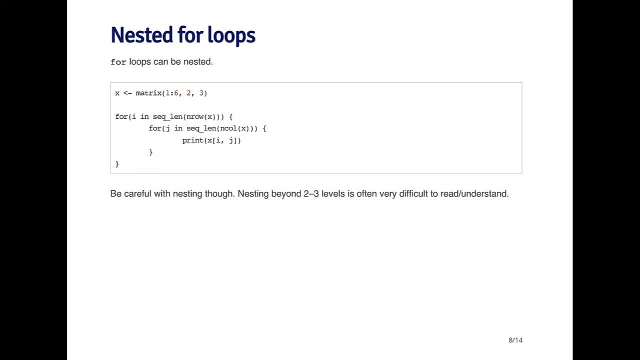 which in this case happens to be the number of rows in x, And then it creates an integer sequence out of that. So this particular matrix has two rows, And so it's going to create the sequence one to two. Similarly, the nested loop with the j index is using the number of columns to create a sequence. 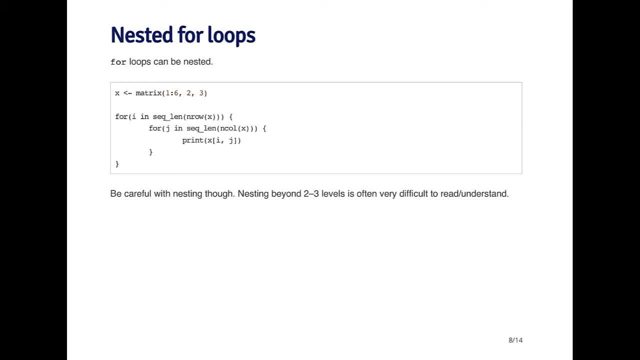 So this matrix has three columns, And so the seek underscore len function is going to create an integer sequence, one through three. So this doubling nested for loop is basically printing out all the elements of the matrix. So one thing to be careful with nested for loops is that it's going beyond two to three levels. 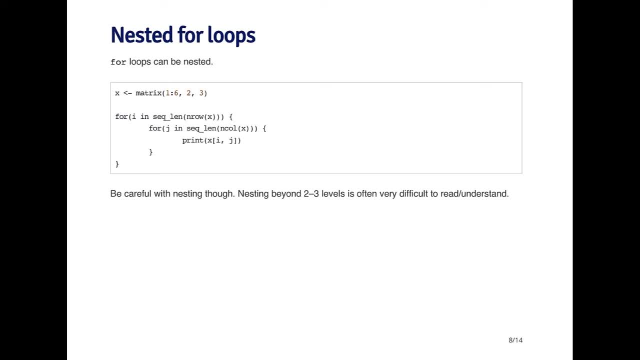 So while it's theoretically okay in R, it makes reading the code a little bit difficult to do, And so if you're reading code that has three or four nested for loops, it gets difficult to understand what's going on. Sometimes that's the logical thing to do. But many a times there's ways to get around that, for example by using functions.